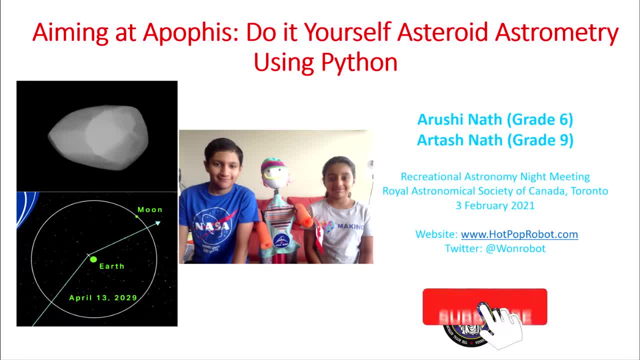 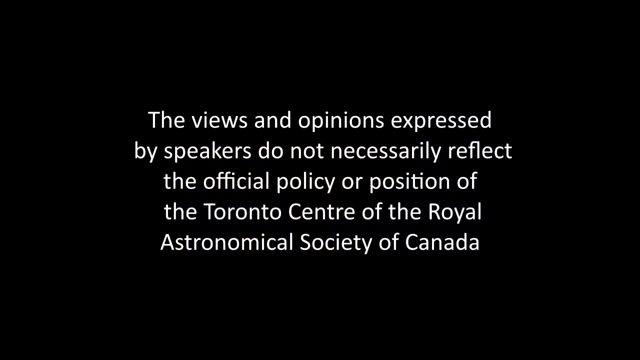 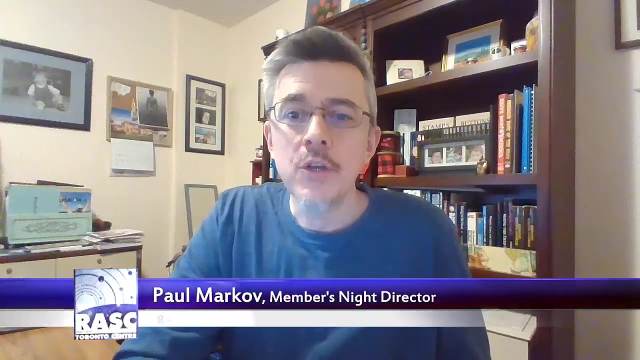 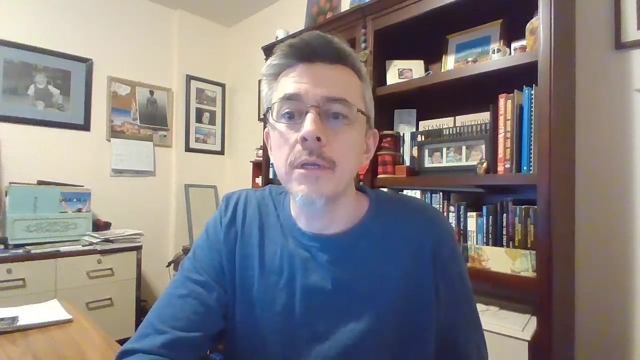 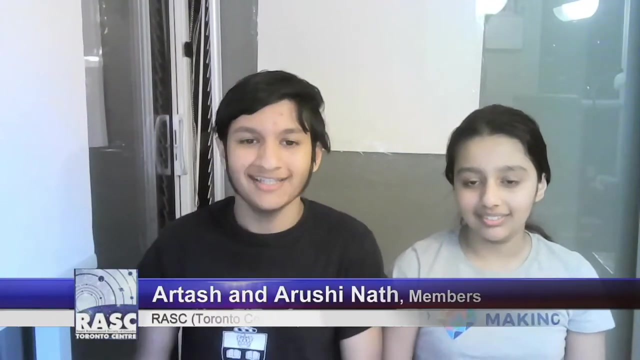 I think we can move on to our second presentation. Artash and Arushi Nath will talk to us about do-it-yourself asteroid astrometry using Python. Go ahead, guys. Thank you, Hello everyone, Good evening. My name is Artash Nath and I'm a Grade 9 student here in. 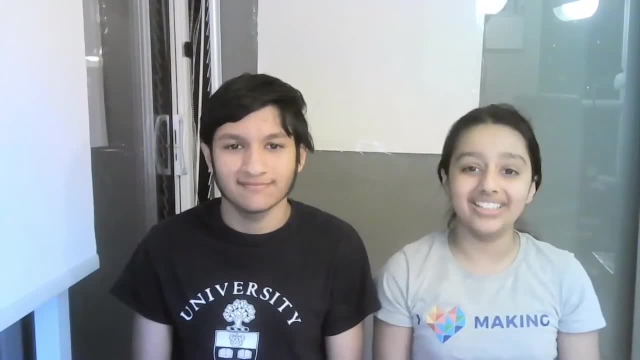 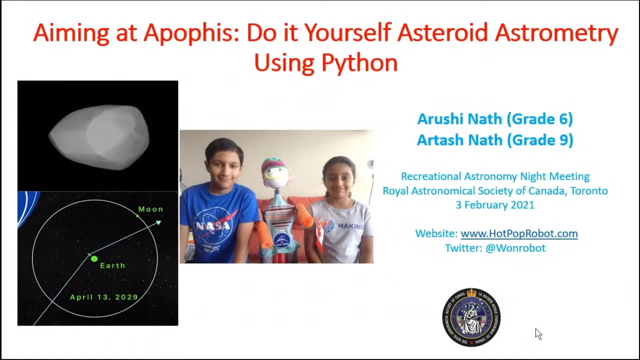 Toronto. Hello everyone, I'm Arushi and I'm in Grade 6.. Today I'm going to talk to you about do-it-yourself asteroid astrometry using Python. So I love asteroids. I'm going just in there. Asteroids are. 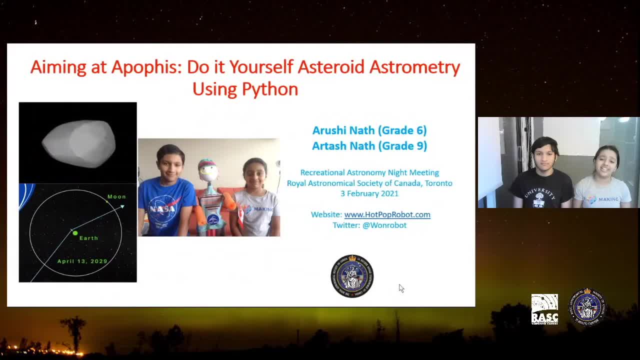 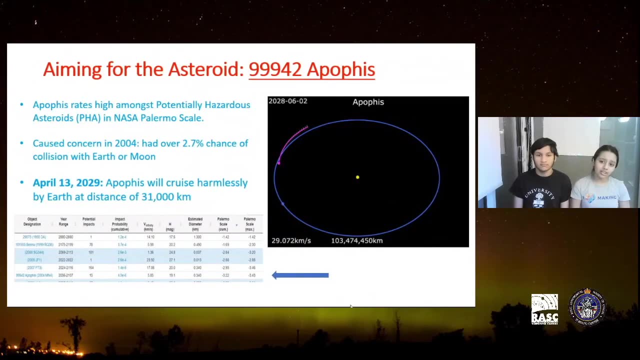 objects which, just like planets, like the Earth, orbit around the Sun. Most asteroids are found in between Mars and Jupiter, But if planets aren't, sometimes they go beyond that limit and sometimes they can go very near the Earth. So when they go near the Earth they're called near-Earth. 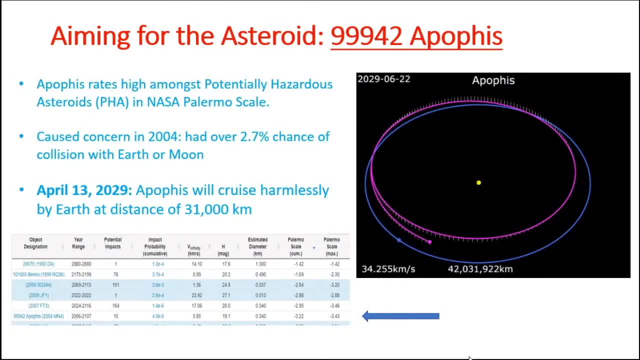 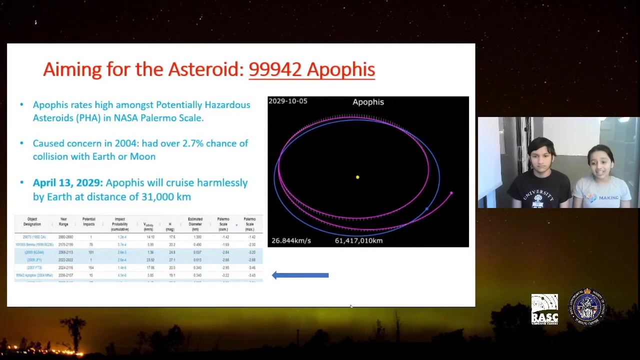 asteroids, But if they go very close, they're called potentially hazardous asteroids And it's very important to keep observing these because sometimes it's possible that one of these asteroids that will intersect with a path of the Earth. So I got very interested when I found this out and I wanted to 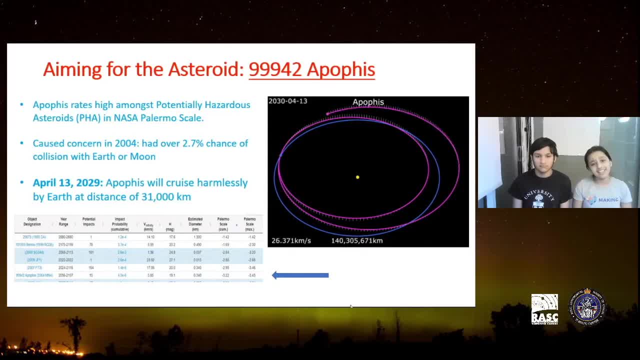 learn as much about asteroids as I want, as I could. So I decided: why not? Why not actually look at asteroids and try to find the most information about them, like their velocity, for example? So I decided to start with 99914, Apophis asteroid. Why? 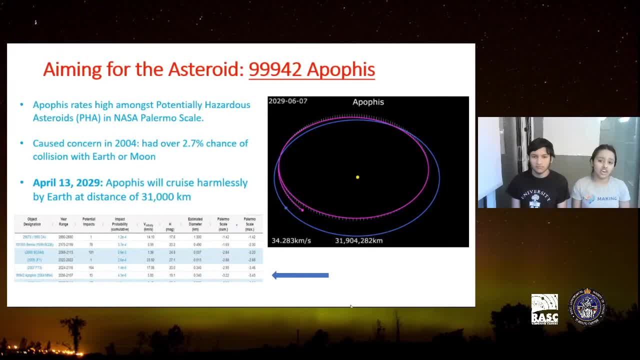 Well, first of all, Apophis is one of the potentially hazardous asteroids PHAs, And in 2004,, astronomers detected over 2.7% chance that this asteroid would go device-prechen over space. If I could say, there's one possibility. 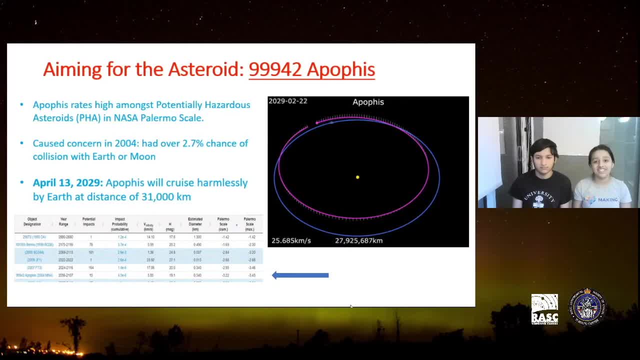 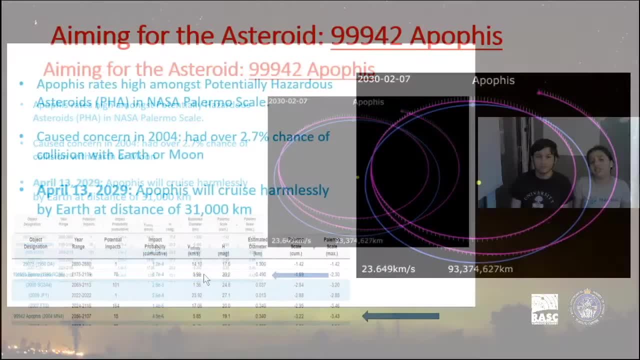 Uh-huh. One probability is them. More than that, More than that. And then yağ. what is your next point, estem, por favor, can you hear me say this? Okay, will intersect with the earth or the moon, and nine years from now, in 2029. 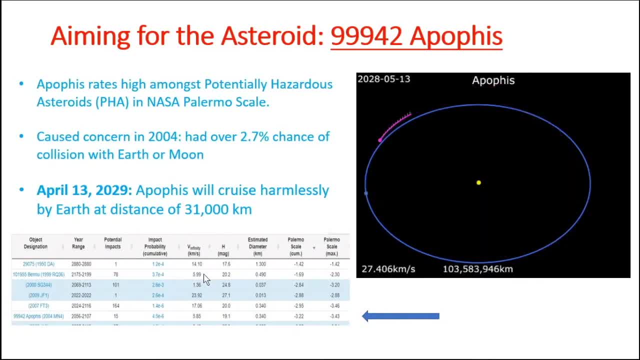 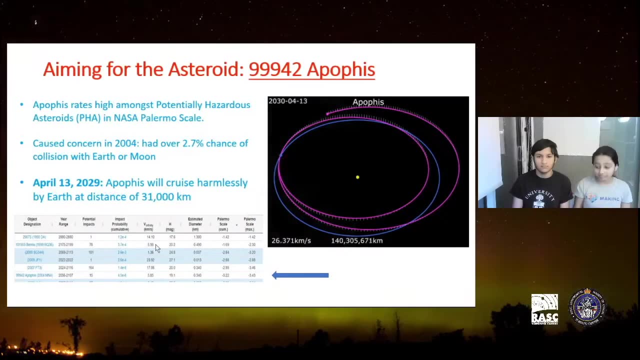 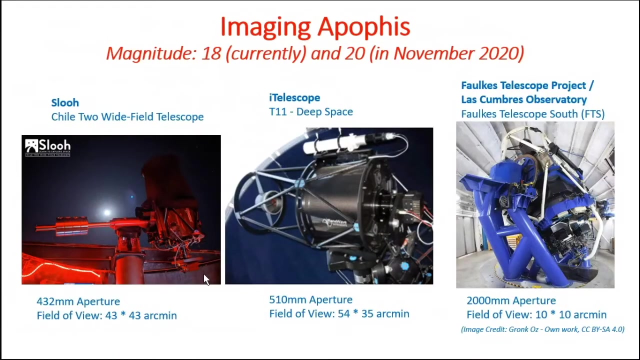 the apocalypse will go very close to the earth- just 21 000 kilometers, so that's even closer than some of our satellites. so i wanted to take first step to getting the data about this asteroid was to actually look at it. so for this, unfortunately, i could not use my own telescope that i have in my home. 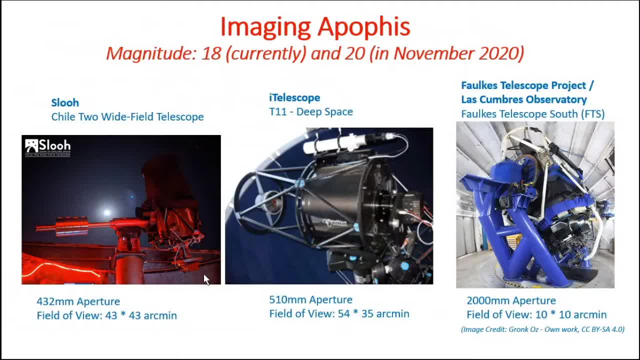 because its aperture is around 15 centimeters. that meant that it was not enough to capture enough light to see them object, because this after asteroid is quite good right now, like it's around 18 magnitude and when i started this project in november it was magnitude 20. 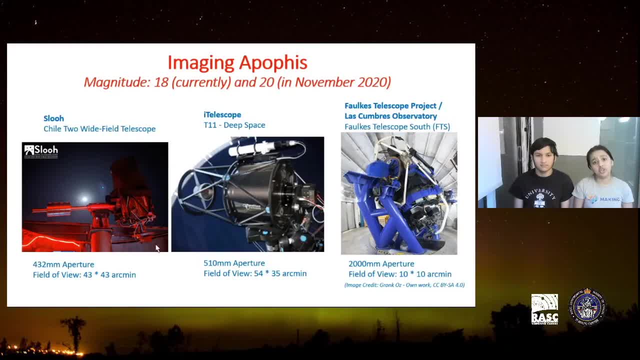 so i needed to use a robotic telescope, which means from my home i can control the telescope very far away. so i started doing some research. the first telescope i found out was from this little website. there they had a chip of telescope called chile 2 and it really helped me getting. 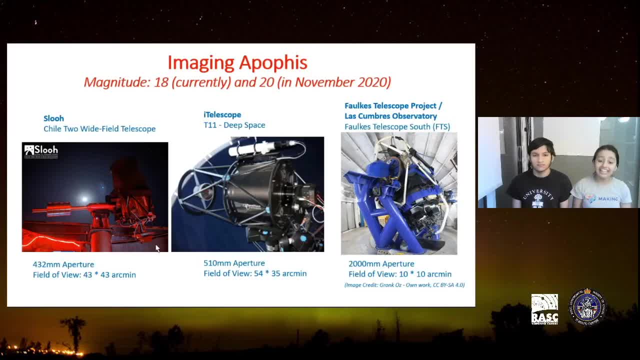 the basics of how to operate a robotic telescope and i learned a lot of new things. but unfortunately, when i ended up at the office, i was not able to see the asteroid because still the aperture was not enough for the three centimeters, so i needed to look for a new. 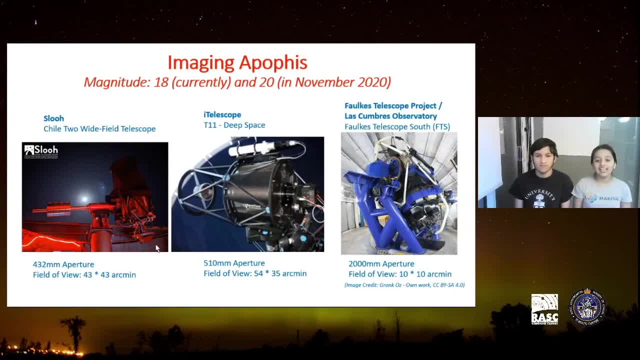 telescope. i found out about itelescope where they gave many telescopes and you were able to book reservation. i looked at a t11 telescope- deep space- but unfortunately here it was not. this was still not enough for a chip, so i knew i knew i needed to get a big change so i can look at the asteroid. 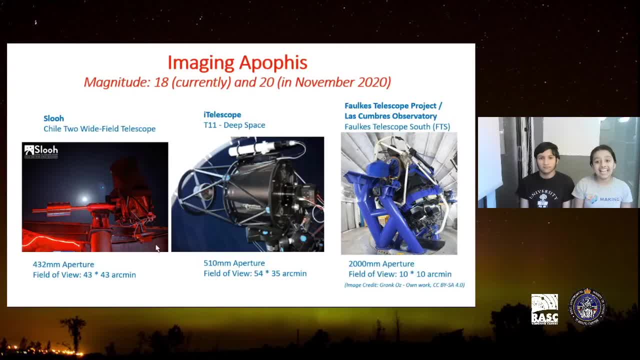 that's when i saw the volks telescope project from the last converse observatory. their telescope had a aperture of two meters, so that would be enough for me to take observations. so i contacted them and they generously gave me access, a couple hours in my day, to their 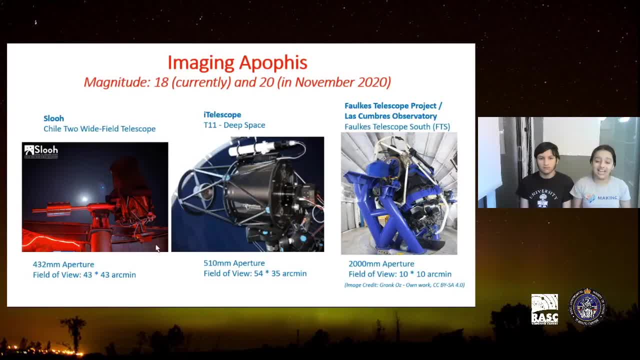 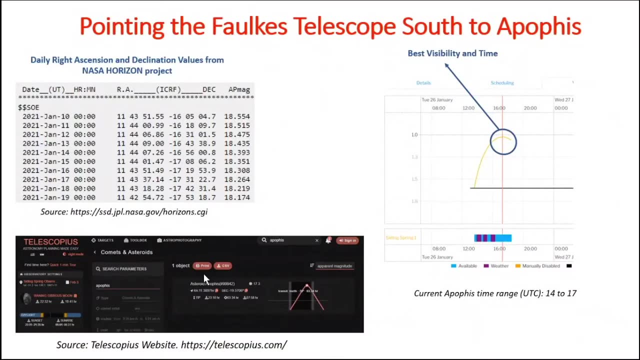 telescope when they heard about my project and how i wanted to learn more about asterism, especially a box. so now i had a good telescope to take observations. now it was time to actually take the picture of a box. but for that i would have to know where to look at, because i can't just tell the telescope. 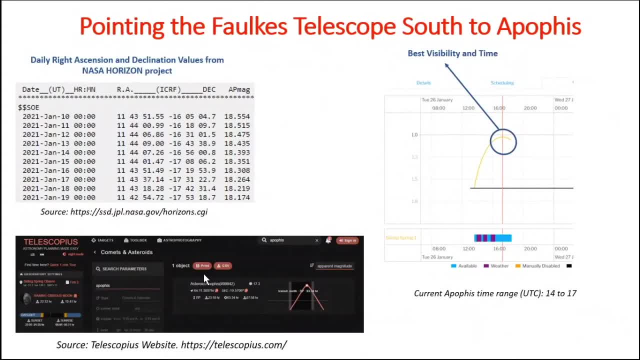 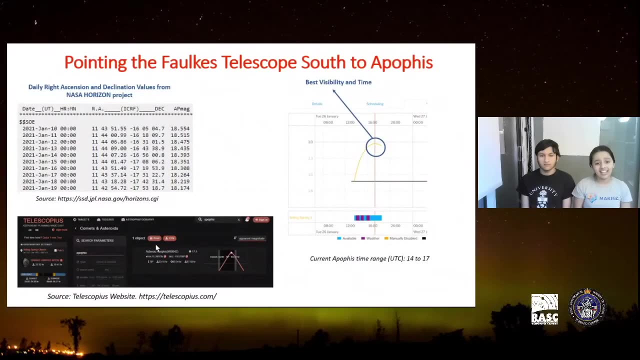 to point at the box, it will have to be more specific. so i went on the telescopius website. they gave me the right ascension and declination of my hypothesis asterisk, but unfortunately they only updated it every day and as the telescope had a pw, relatively small, 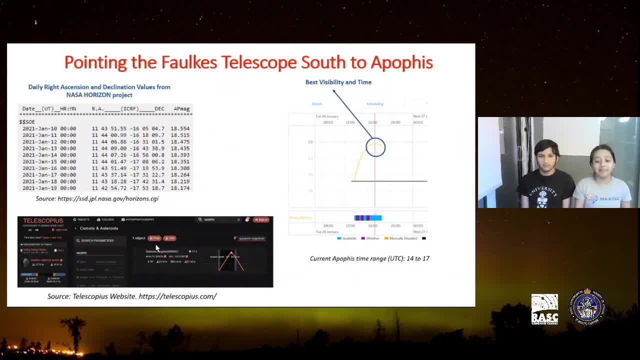 of 10 by 10 arc minutes. it might have disappeared by the time i actually get them from these coordinates. so i needed to get more accurate rate, ascension and declination coordinates. so here i found out about the horizon structure and here they gave me daily. they gave me daily price, section and declination. 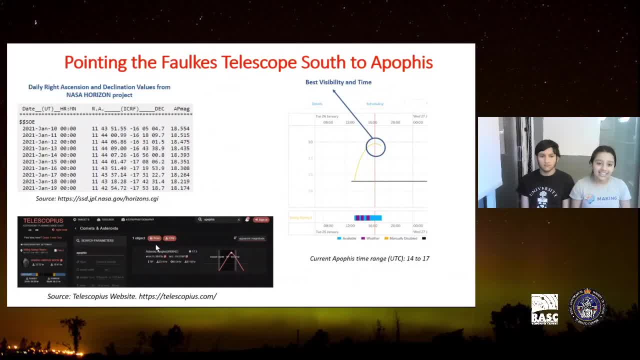 coordinates of the asteroid. so this was good. now i wanted to know when exactly should i take the observation, because i need to know when is my, when is the asteroid going to be above the horizon and where it's going to be below the horizon. so here i have two options: telescopius, boot telescopius and the full telescope. 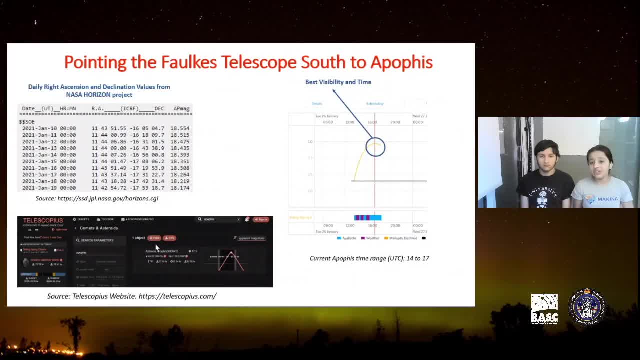 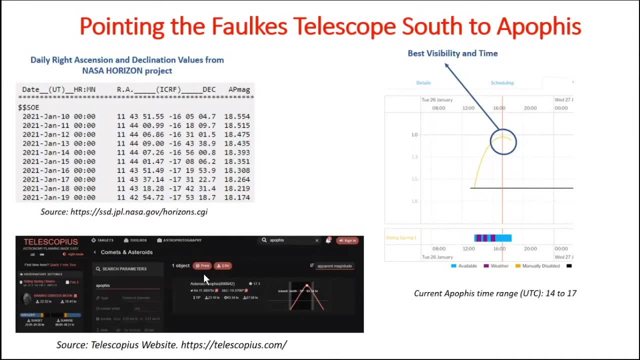 website gave me this data. so, as you can see in the graph, you can see that this kind of like a peak, and the best visibility time was 14 to 17 o'clock utc. so now with this information i could go back to the nasa horizon state project and i could get that exact time. so i hit the observation. 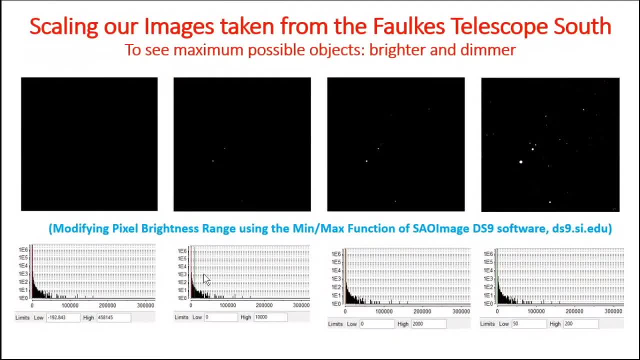 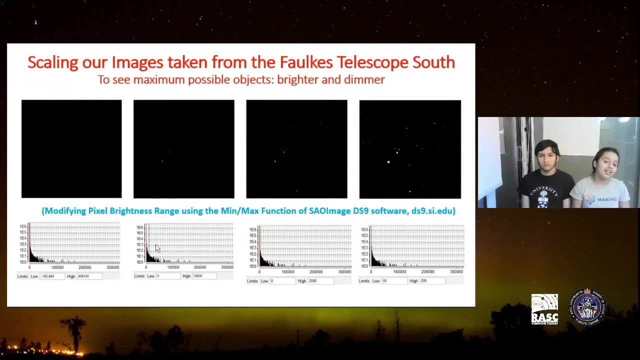 the next step. actually, telescope had got the image, so i had to use a special software to open this image, because it wasn't a normal jpeg or png format. it was in a fits file format. so when i open the image, well, why fits files, why not just a normal image file? the thing is fits files. 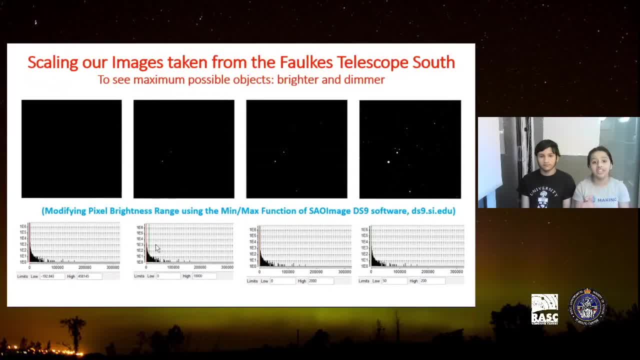 have more than just the image. it also has lots of data about the image, for example, which telescope did the image, when did i take the image, what camera was used to take the image, and so on. so this would be useful later on. but when i opened the image, i didn't. i didn't find multiple stars or objects, as i expected. 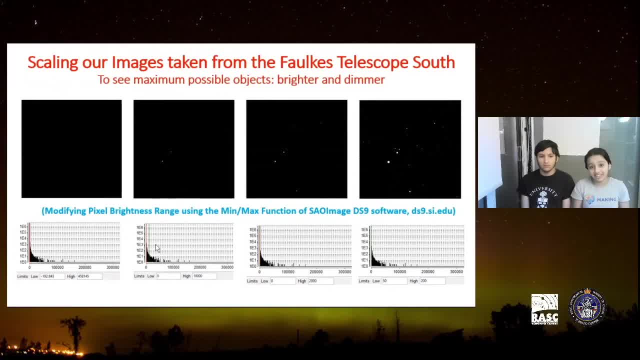 i found a black screen which won them out. so i was really surprised. i thought: did i underexpose it? did i overexpose it? but i soon found out it was nothing to do with that. the thing is, i had to scale the image before i can use it. what does that mean? well, when i get 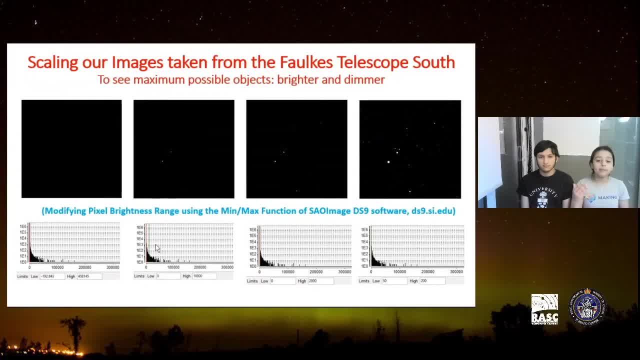 the image it's, it's um the pixel, the pixel brightness. it has a high range, so it doesn't take higher brightnesses better than lower brightnesses. so i had to decrease this range. so, as you can see in these four figures, the first image is black and then slowly you can see. first, 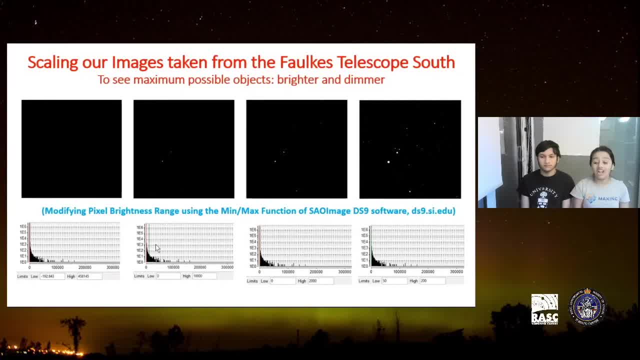 right object and then on the last figure you can see lots of objects and actually if you look at the four bottom graphs you can see in the first one it's from minus 200 to almost half a million is a range of the brightness that that was too much. and in the last one you can see it's being reduced. 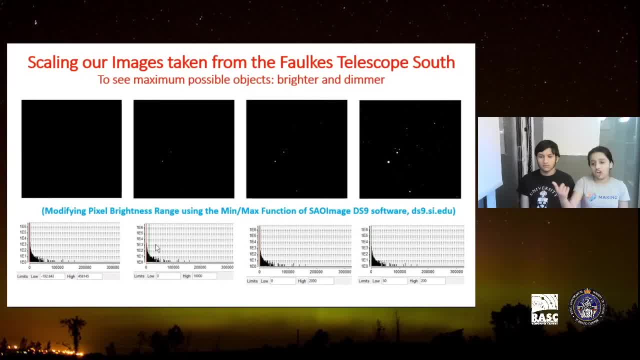 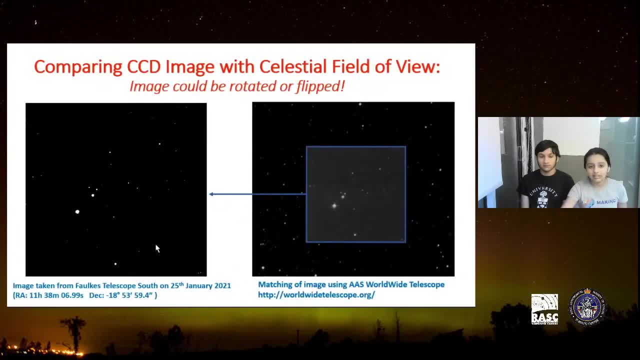 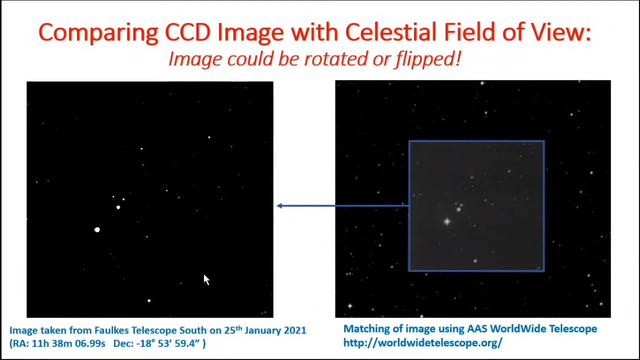 to 50 to 200 and the top image was gone. so now it finished here in my image. it was time to actually start. so first, what i did is i inserted this image into a part into the worldwide telescope, if a software, and i was actually able to see the image in the whole sky, so it just gave me. 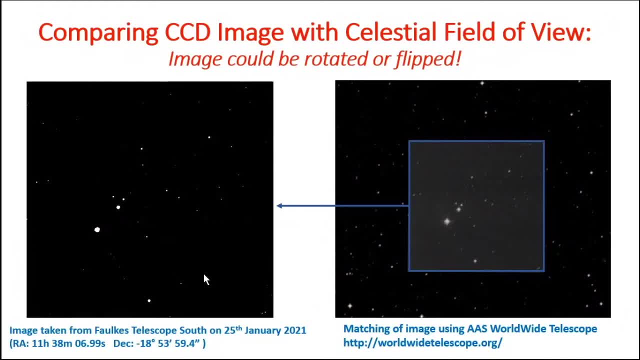 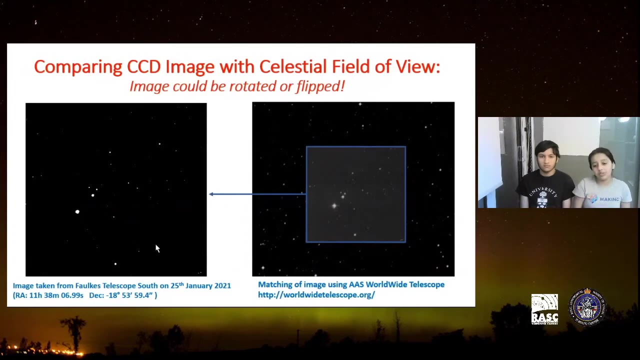 this told me something, two things actually. the first: it verified that to pin the right right section and definition coordinates and fill in the telescope related the image. i could verify it with this software. and it also told me because the thing is when i get the image from the telescope it sometimes is flipped or rotated, so this would tell me what was the. 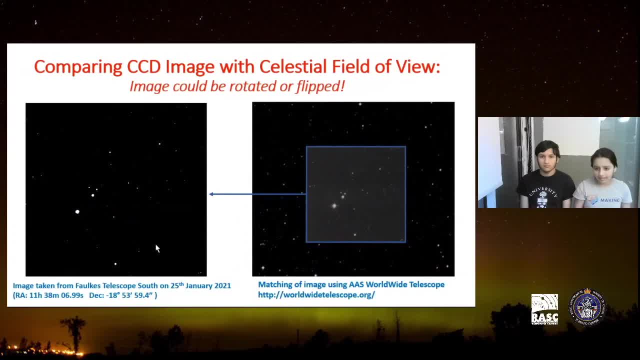 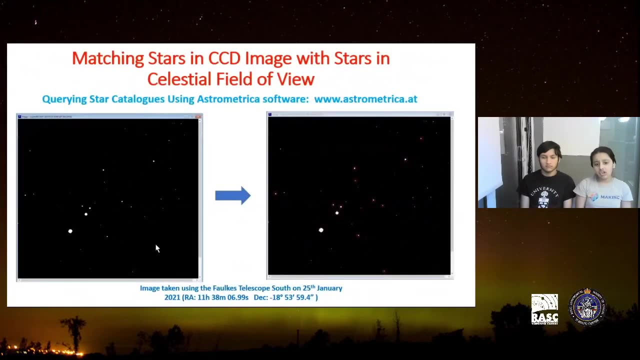 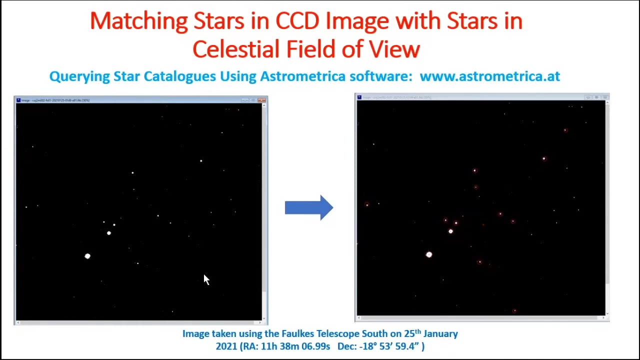 rotation or flipping of this image. so, but if you look at this image, remember my main goal was to look at the fossils asteroid, but how could i know which of these images is the fox? so i had to do something about it. so i decided to actually overlay the catalog on top of this image so that 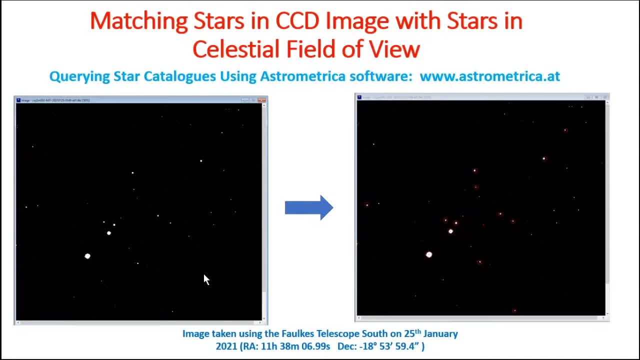 because the thing is, this catalog would tell me stars, but i was not interested in stars, i was interested in asteroids. so it would be able to remove all the stars from the image or tell me what the stars were. so i knew that none of those objects were the asteroids. so, as you can see in 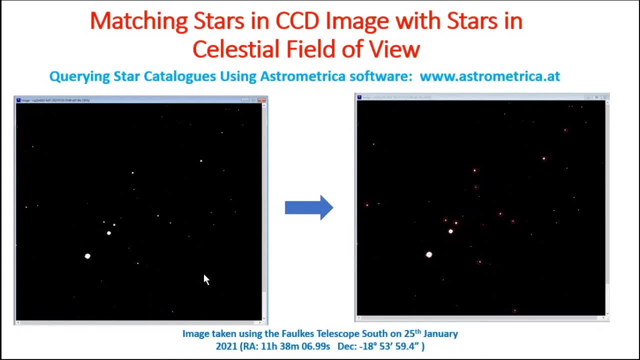 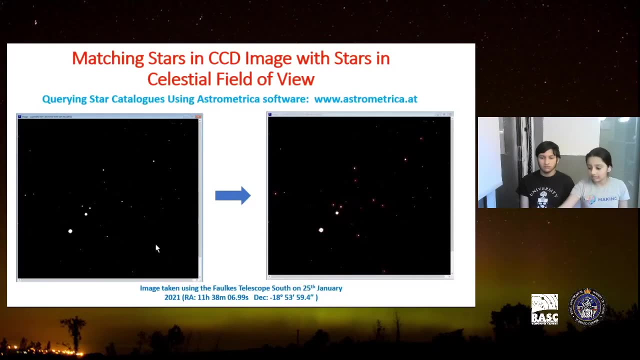 the second figure there is a red circle around some of these objects. that meant that these were recognized stars, but the problem was there was still some for many objects that didn't have red circles. how many? which one it is? so i overlaid the minor planet center database. 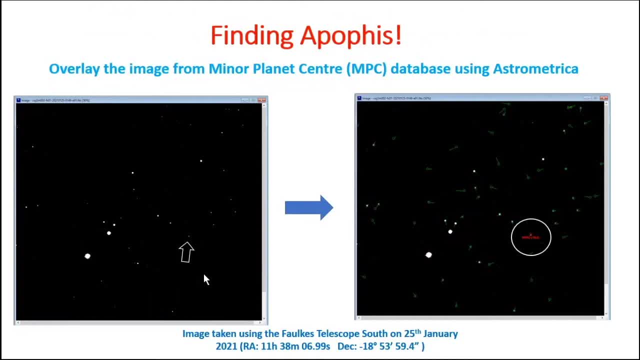 which told me about asteroids and i was actually able to find it in Fußfels Земling ver반aven, 99942 Apophis asteroid inside the image, as you can see in the second figure And we can see it's in the third line of asteroids And if we verify in this image, 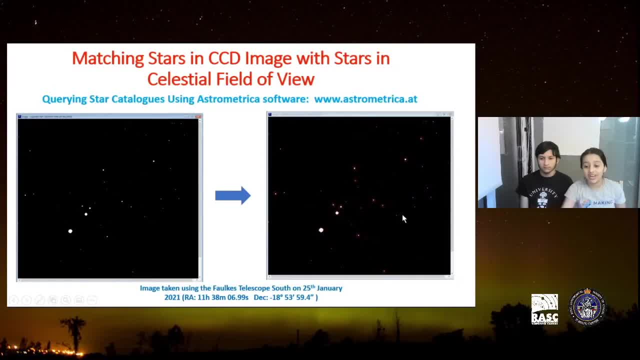 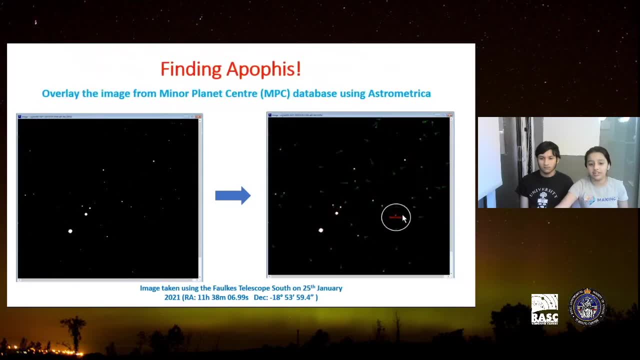 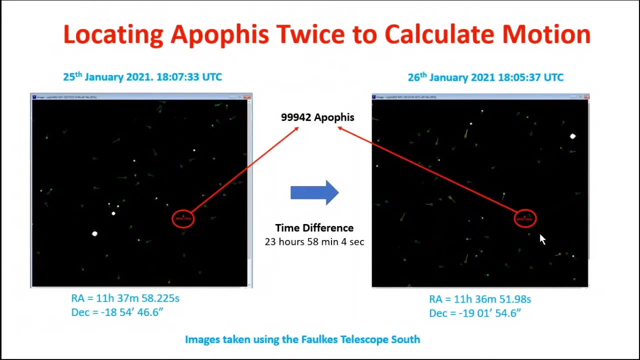 we can see that the third one does not have a red circle on it. so that's verification, because I'm just verifying that it's the asteroid, because it wouldn't have a red circle. So I did the exact same process with the second image of Apophis that I did the next day. 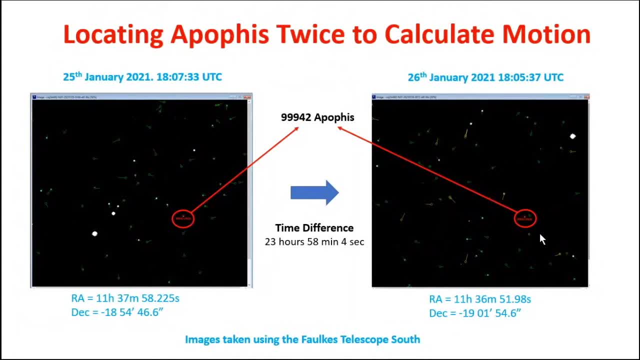 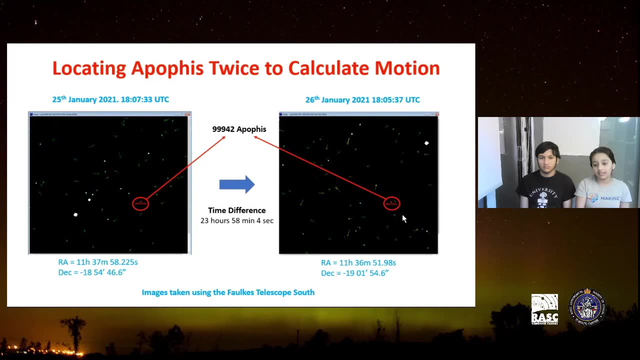 because I wanted to find out about the motion of the asteroid, which meant that I needed to find two images so I can see the difference of the right assumption and the declination point. So, as you can see in this image, the asteroid, in both the images. 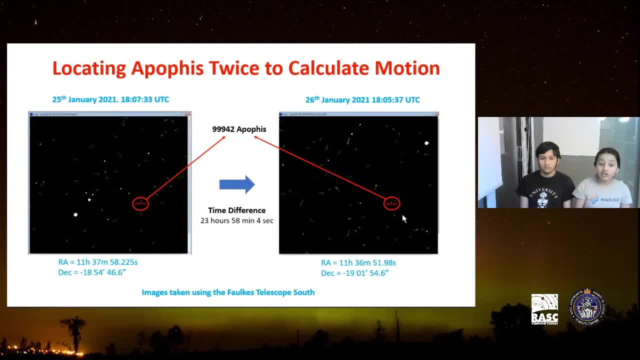 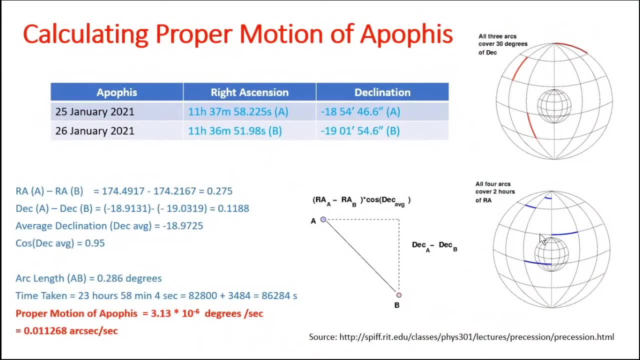 taken a day from each other and the exact coordinates of this asteroid. That was actually calculating the motion or proper motion, because we're only seeing a 2d image, So we can only see the minimum distance the asteroid traveled, because they might have traveled in the third dimension but we wouldn't know. 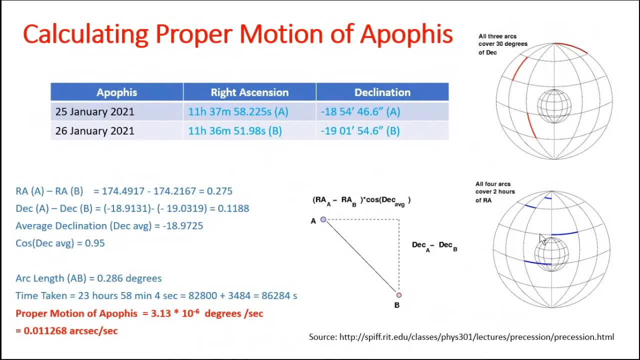 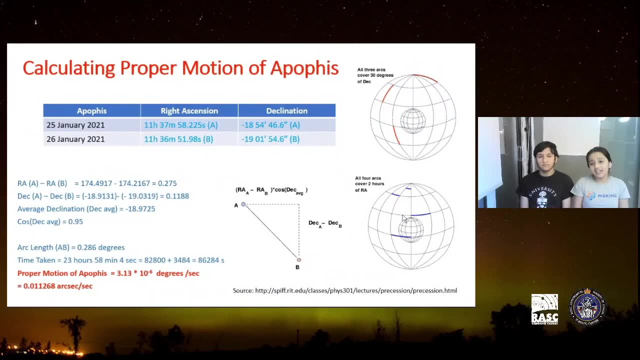 So finally I used Pythagorean matrix, the first side. so basically the change in declination was quite easy. I just subtracted the two in arc minutes. But the right ascension was more difficult, because the right ascension actually the distance between right ascension. 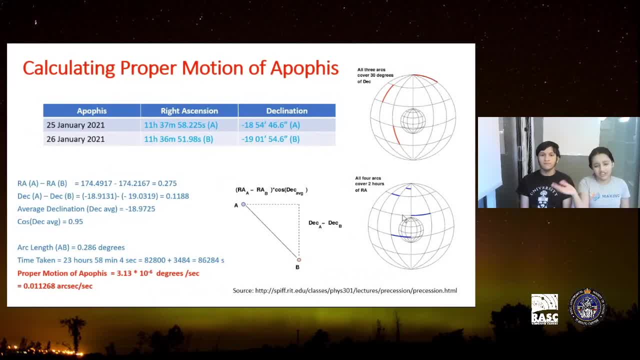 actually changed depending on if you're near the equator, where the right ascension distance would be bigger, and if you're near the poles, where it would be much smaller. So I actually needed to use the declination as well to find the distance in the two right ascensions. So I found the 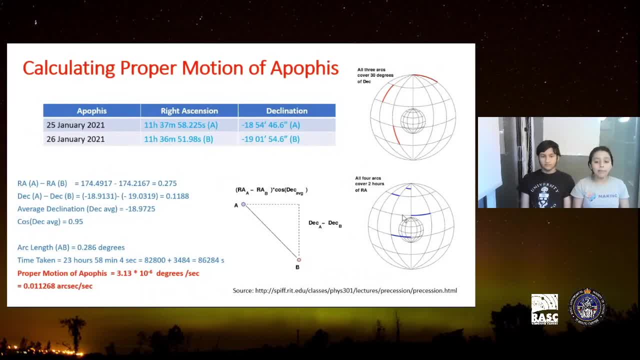 formula which, basically, I multiplied the difference in right ascensions with the cost of the average of the two declination coordinates from each image. Then I found out that the proper motion of Apophis was 3.13 multiplied by 3.. 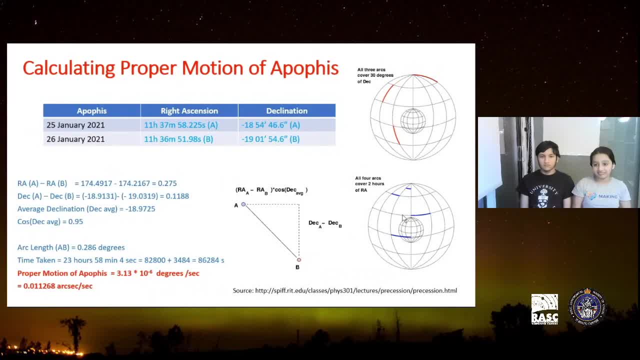 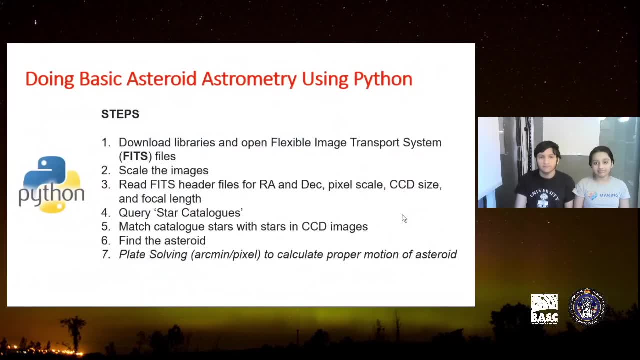 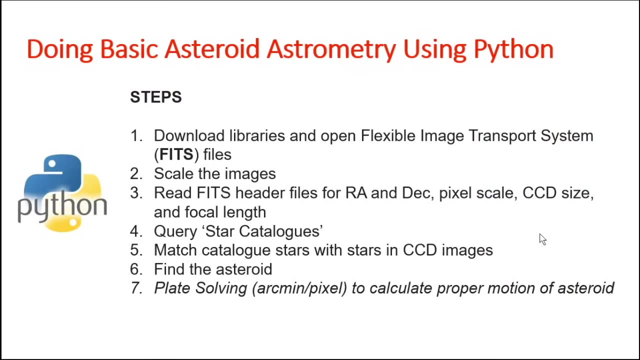 10 to the power minus 6 degrees per second. So now, as I said before, this was a minimum And I'm also actually really interested in Python programming. so I wanted to replicate the steps of using those two images and locating the asteroid in those two images, but using no. 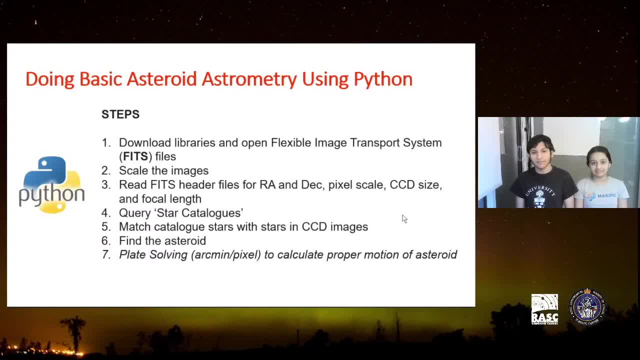 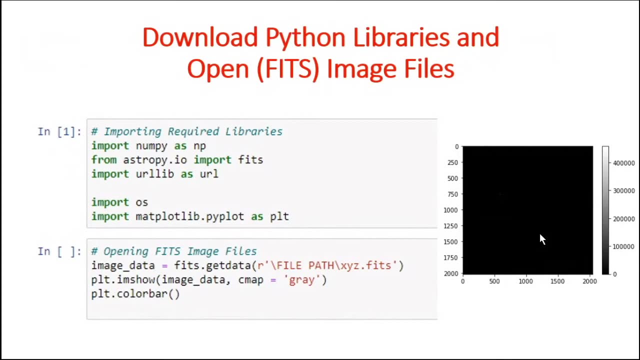 other software, just using my own Python programming skills. So there were seven main steps in Python to finding the asteroid in the image and I'm going to go through six right now. The first step was first importing the libraries I'm going to use in Python to help me with the 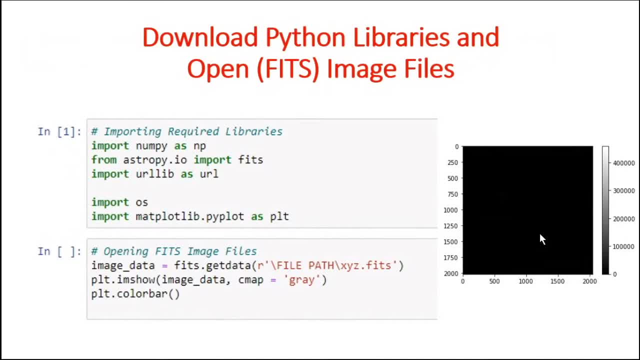 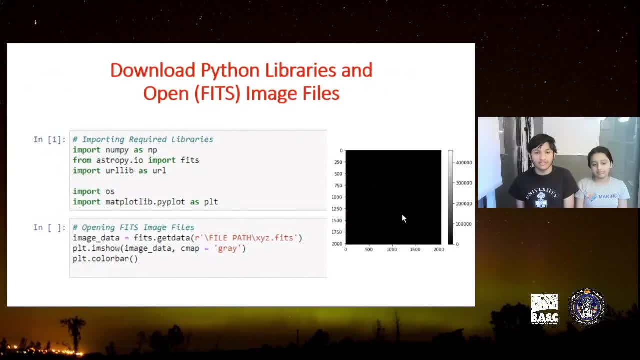 image data Libraries are just like functions or tools I can use inside my code to make the process easier. So I opened the FITC file using a library called AstroPy, which is really useful for astronomical data, and I made a couple of changes today. 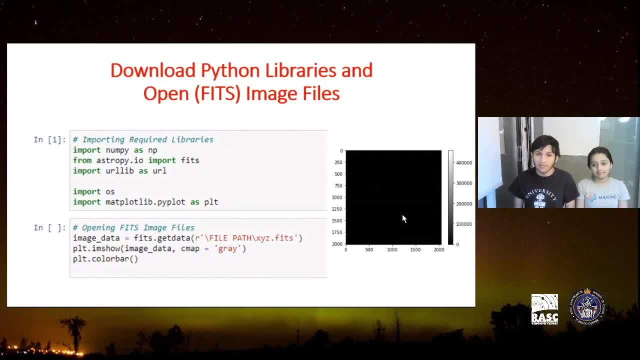 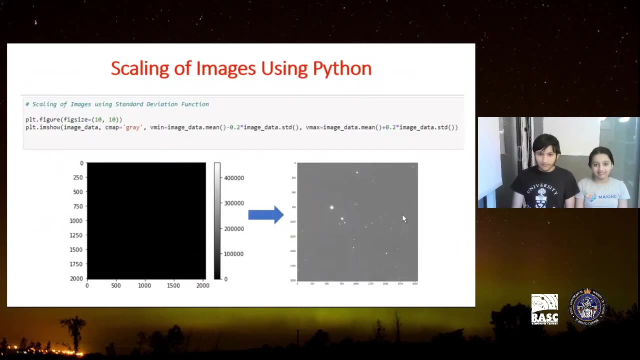 displayed the image, but with that's been read by the 555 on the right. and once again, just like arushi said earlier in the presentation, i also got a black screen with very few stars, just one dim object in the upper left. so my second step was to scale the image, the pixel values inside. 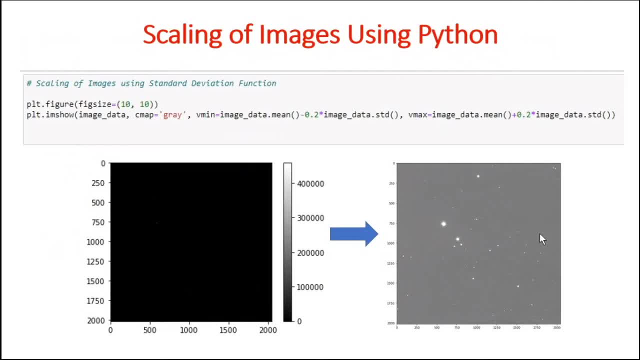 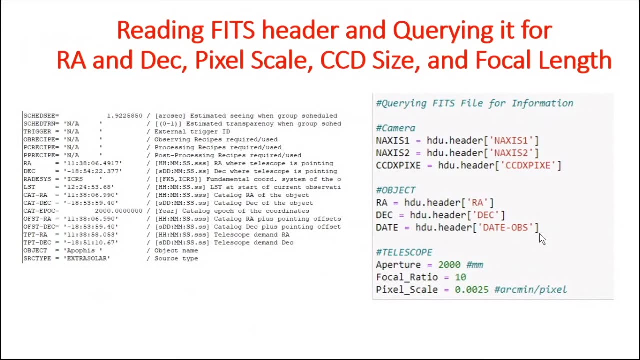 the image so i could actually see objects inside it, and i did this based on the standard deviation and the mean of the image. so the right, you can see the scaled image, which has much more objects inside it. third step: so i needed more information on this image and the fixed file, as arushi explained. 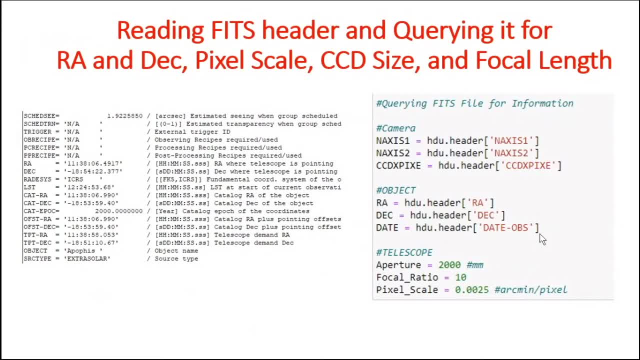 before is not like jpeg. just it doesn't just store the image, it also stores a header that has a lot of useful information about the image, and there were four things. i used python to extract these images from the fits file. the first one was the right ascension and declination of the center. 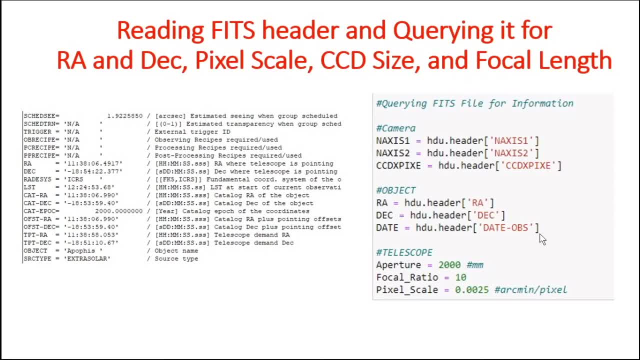 point of my image. the second one was the pixel scale of each pixel in the image, and the pixel scale is really just the size of each image. the size of each image in degrees. for example, if our camera was taking a 10 degree by 10 degree image and had 100 by 100 pixels, 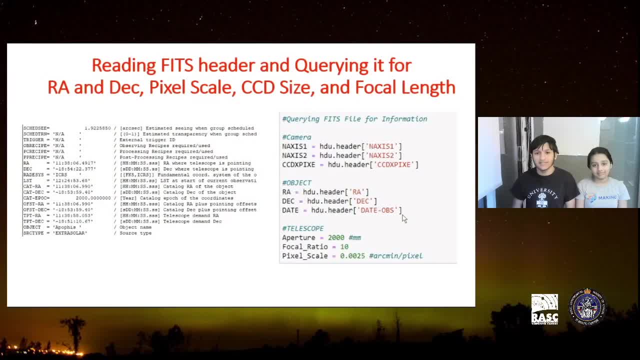 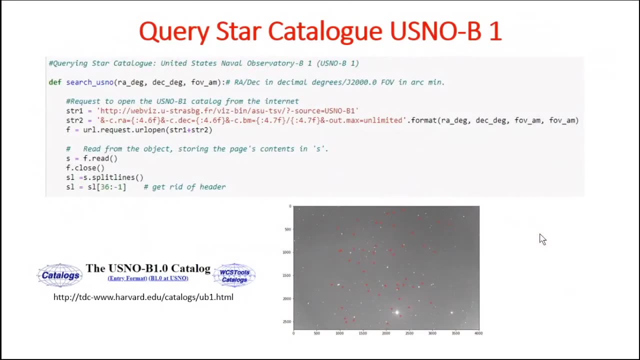 each of the pixels would be one tenth of a degree by one tenth of a degree in pixels. here, further the ccd side, and this was just a number of pixels inside the image and finally, the focal length of the telescope was also. now i had my image but i didn't know what are these objects like before. what is the asteroid? 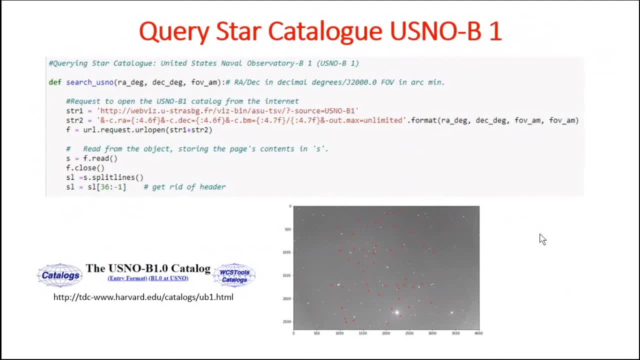 so i queried a star catalog from the united states and naval observatory, which has a huge catalog of all the known stars across the skies. so i took the stars from the catalog that were around in this image and overlaid them onto the image, so at the bottom you can see. 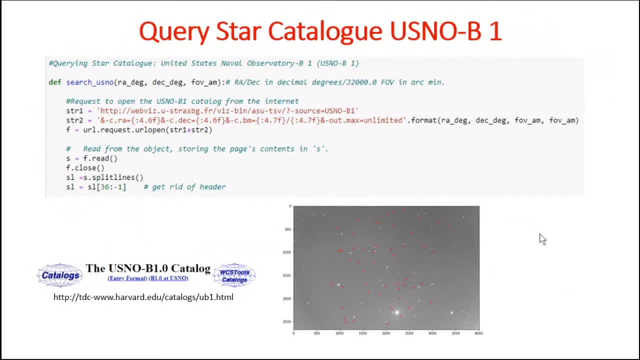 the original image that i took from the previous slide, and you can also see a lot of red circles that have been overlaid on this image, and these red circles are the known stars from the catalog. but you might also notice that they don't match any of the stars on the image, and you know what? 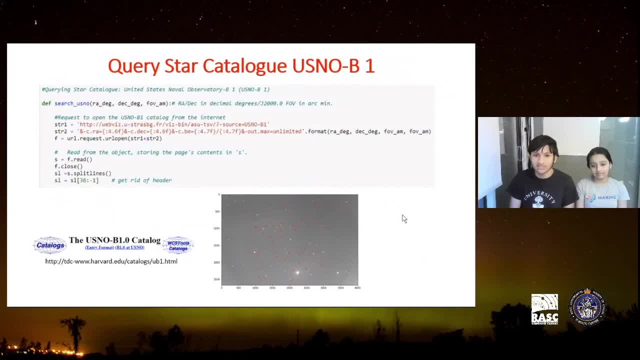 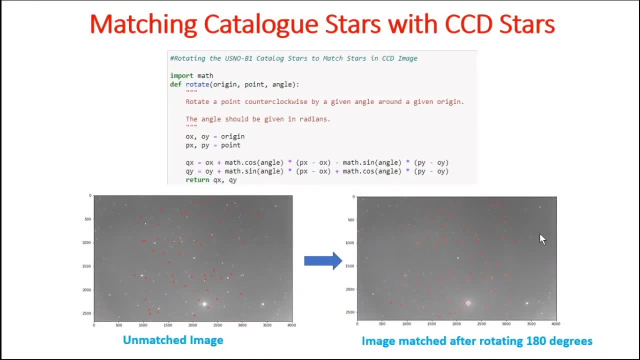 they need to be rotated until they match the stars in the image. so i created another python function that would rotate all these small circles until it found the best fit. so, on the right after, the program rotated all the circles by 180 degrees, which is just a flip, all the red. 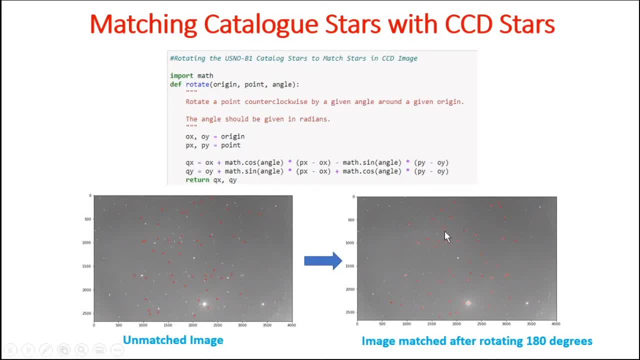 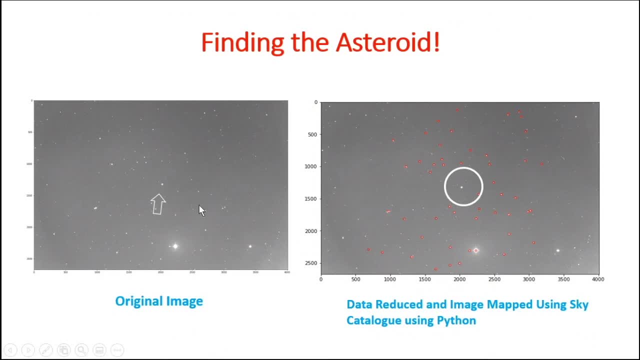 things overlay on most or on a lot of the stars in the image. so here's the original image i had taken from the left and on the right is the image, but it's overlaid with the star catalog, known stars. and here we go. on the center we see our bright object that isn't surrounded by a circle. 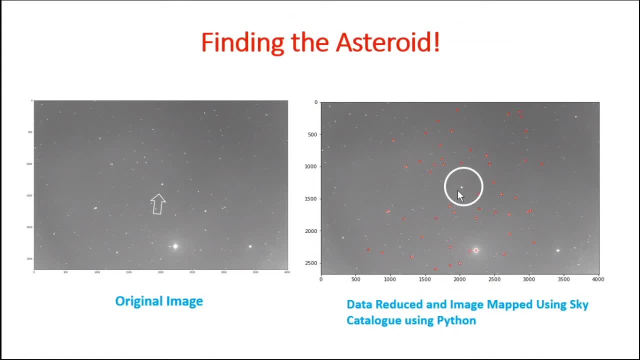 and that is our actual. so i did the same process with the second image. so i was able to locate the after using my python program in both the images and i did the same process, the same process. Formerechad was collecting the distance between these two of the aston yesterday and got the. 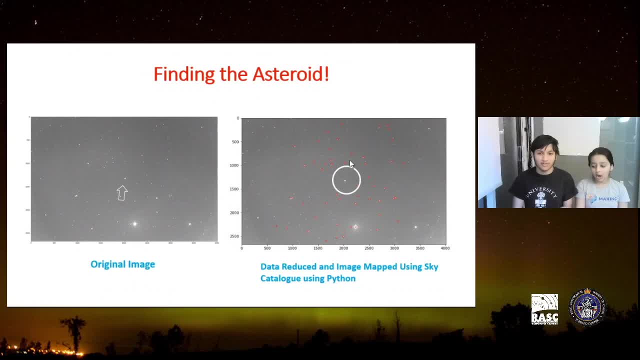 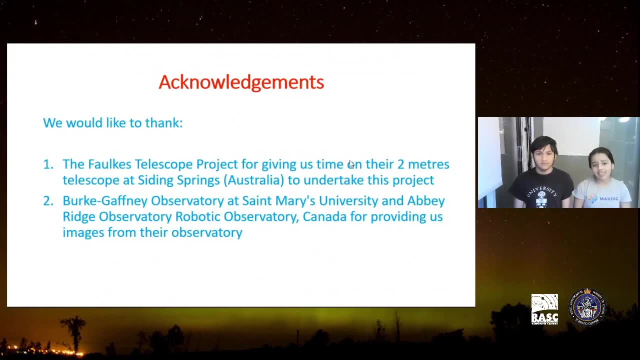 same speed of theenoid as we did using the actual method of the same function. so this project wouldn't have been possible with without two. first is the actual bug chill school project, which gave us time at which actually we were able to get the actual images. 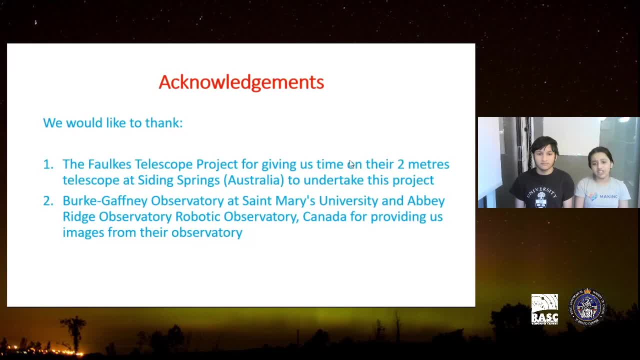 so we can perform all this analysis. the second is the burg gaffney observatory and the answer to this loser guard alles at the ridge observatory, where we were able to get test images from their observatory. thank you, i hope you enjoyed our presentation. i'd be happy to answer any questions if you have me. 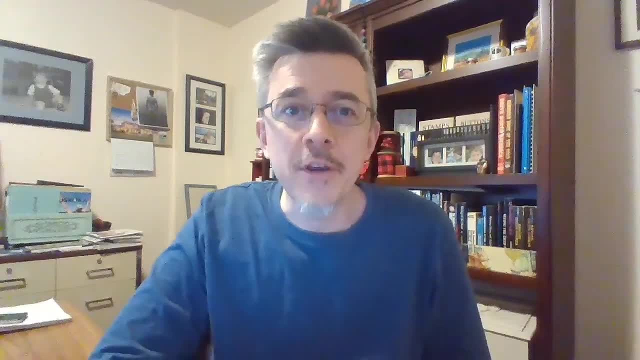 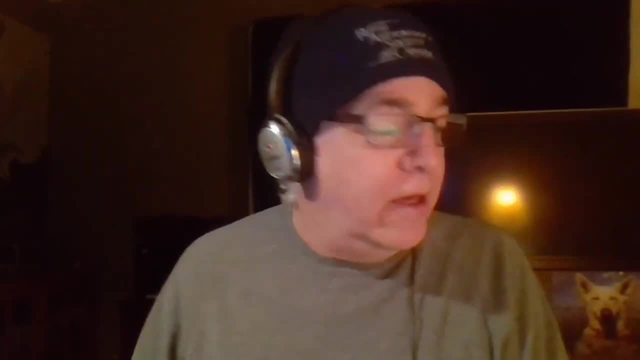 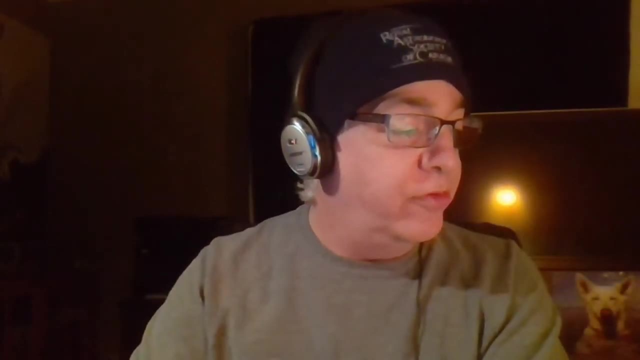 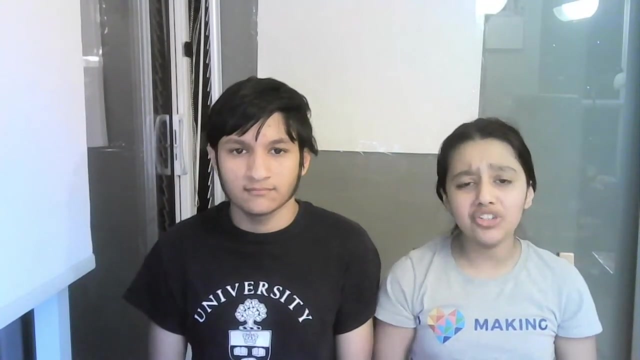 hey guys, this is amazing stuff you're doing. you're on your way to turning professional congrats. let's go to word. any questions for the guys: hi, um, one question from blake. um, for uh, ruthie, uh, did you use uh fitz liberator to uh stretch and scale the image? actually, for scaling the images i used. 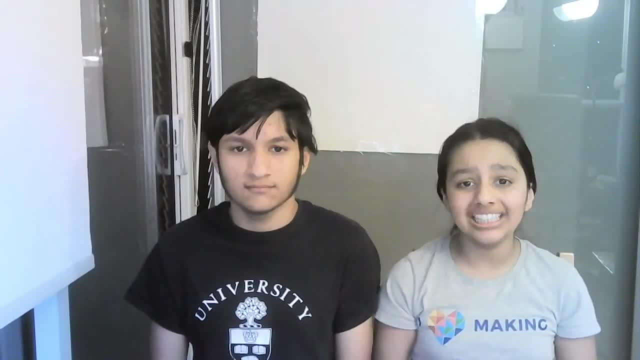 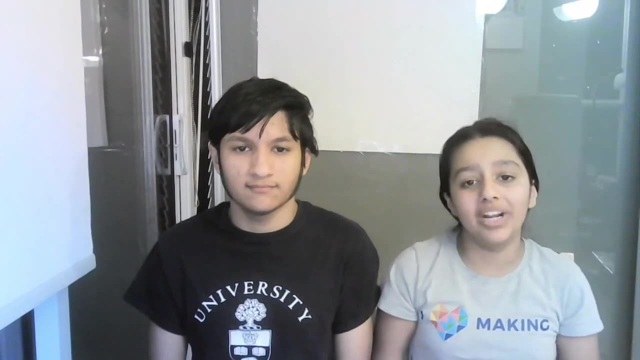 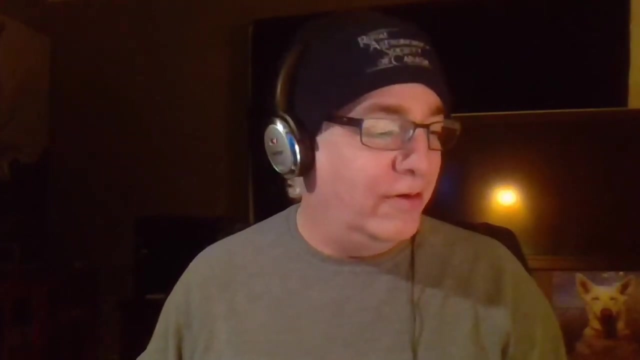 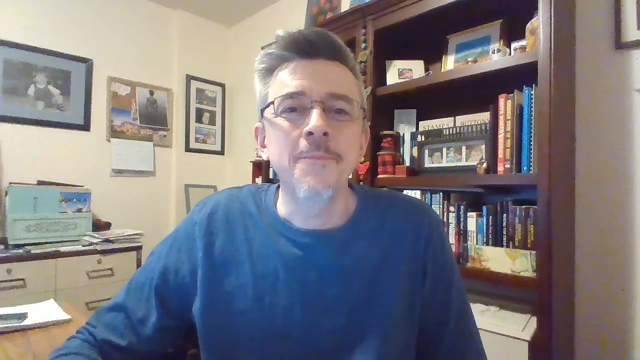 a software called sao image ds9. so i imagine many softwares are possible that, but that's to when i got one. fair enough, jaded your uh. your skills in coding uh, artash are are pretty impressive. well done, okay, no more questions. no more questions. okay, thank you. word uh, thank you.